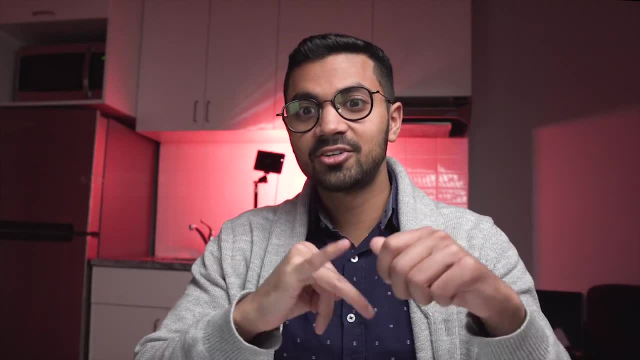 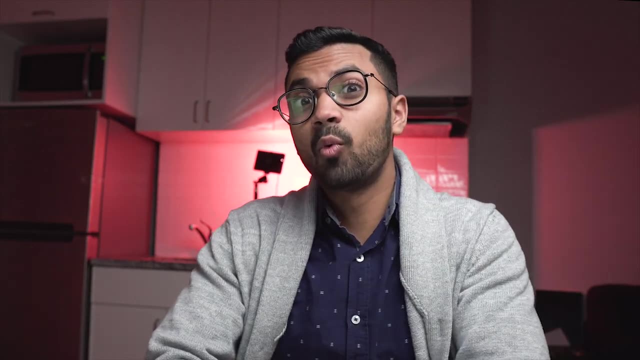 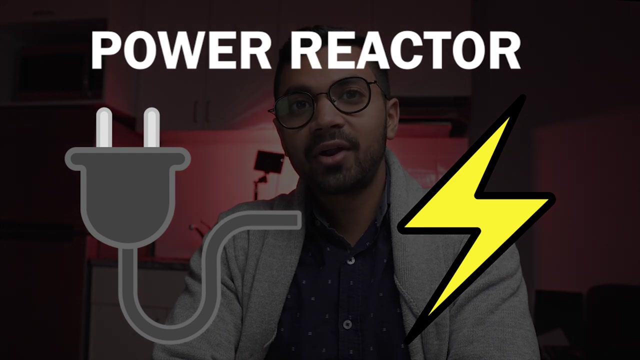 produce clean energy. They produce radiomedical isotopes, fight cancer, they are used to propel marine vehicles and they're also can be used to create even more fuel for create more energy. So let's start off with number one: power reactors. Power reactors are just. like the name implies, they create energy, lots of energy. They are responsible for creating huge amounts of base load power for nations across the world. In the world right now, there are around 440 operating nuclear reactors. In total, they produce 10% of the world's energy. Now this number is projected to rise to. around 900 operating nuclear reactors by around 2050.. But with the advent of new technologies like small modular reactors, we're seeing that there are potentials to drive down cost, make nuclear power more accessible to other developing nations. Okay, what are the advantages of? 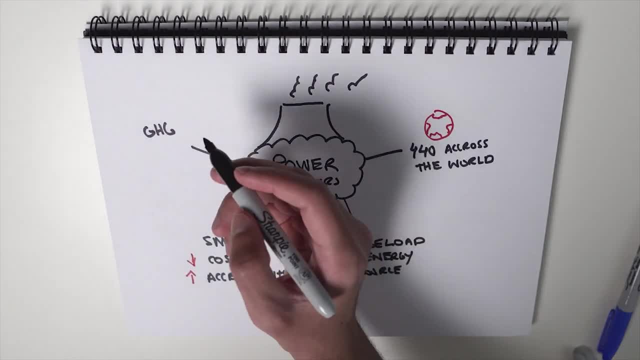 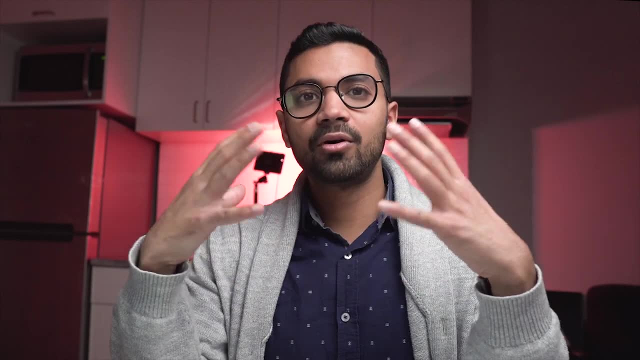 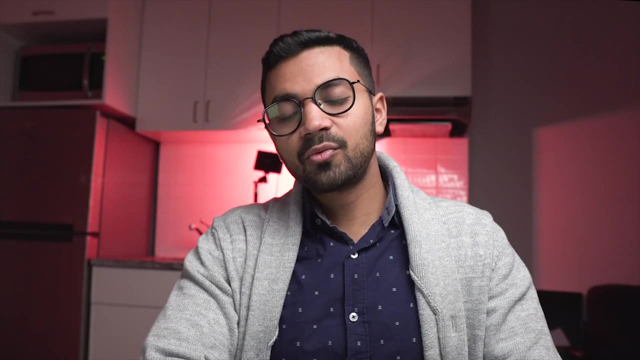 nuclear power reactors: Zero greenhouse gas emissions during generation of electricity. Also, they take up less land. Okay so, reduced environmental footprint and many, many more benefits, which I will discuss in my other videos. Now let's go into breeder reactors. Number two are breeder reactors. Breeder reactors are: 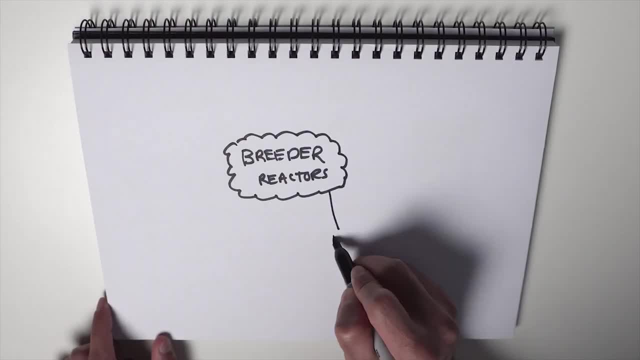 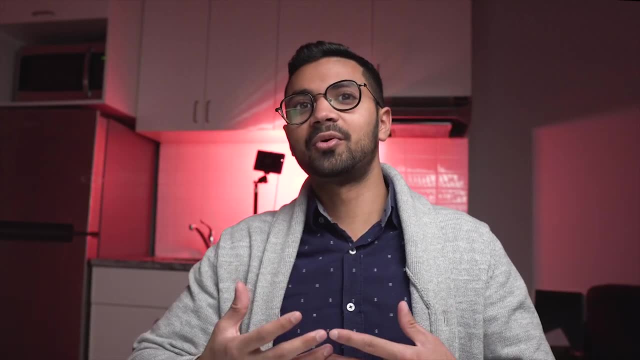 also a type of reactors which produce electricity, So they are power reactors as well, but they're different in a sense where they produce more fuel. So they actually produce fuel as they operate. To give you an understanding of how breeder reactors work, I'll have to give you an idea of how nuclear fuel works. So 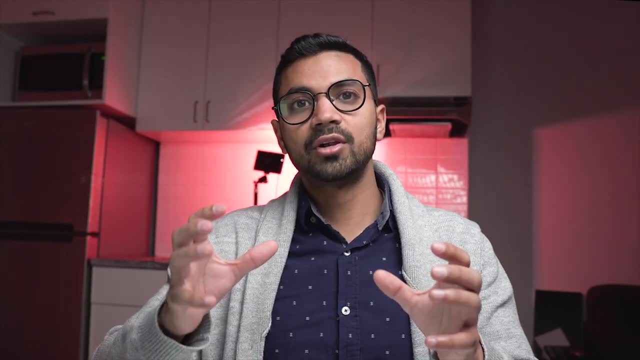 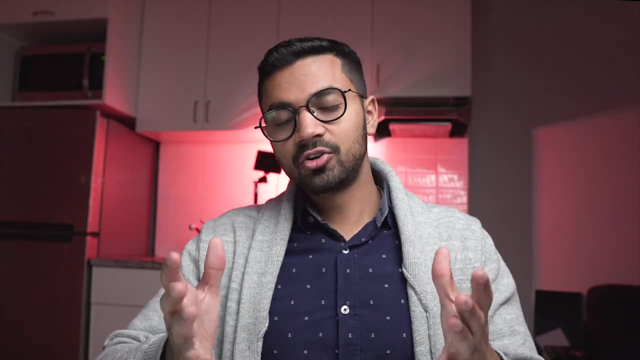 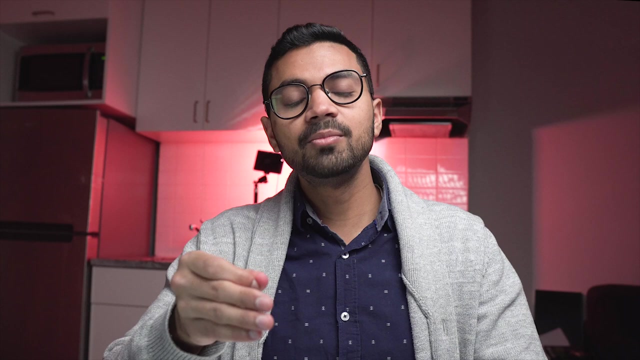 in terms of radioactive isotopes, there are two categories. One are fission, fissionable isotopes and second are fertile isotopes In nature. naturally, the fission isotopes are very, very rare. So U-235, which is a fission isotope only. 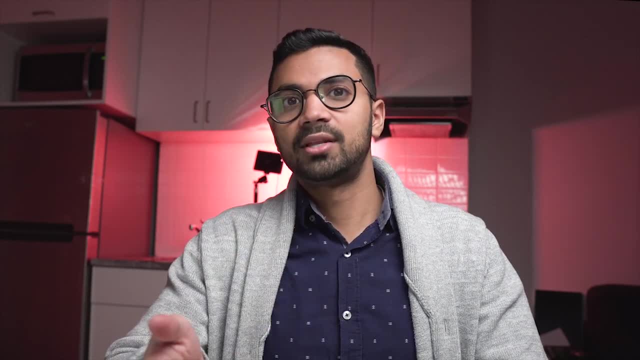 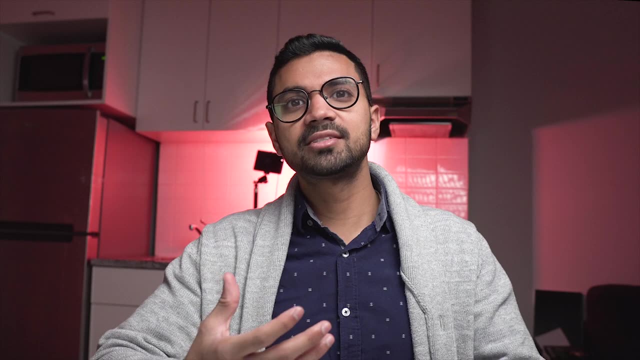 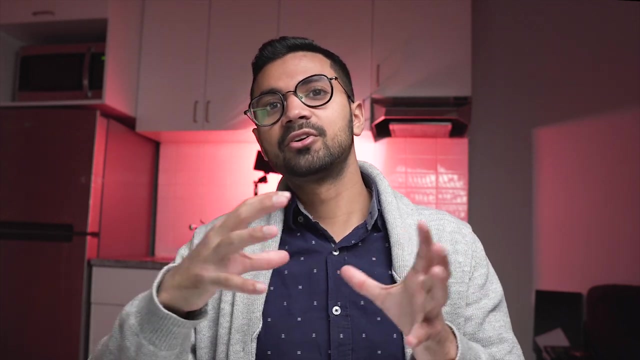 makes up 0.7 percent of the world's uranium. Okay, it's a very, very small, small percentage. And to mitigate that, what, what, the what the industry does is? we utilize an enrichment process. Okay, so we utilize centrifuges which filter out this material and increase the amount. of U-235 in the fuel. It's an expensive process. In the 1950s and 60s breeder reactors there was a lot of interest in this technology because of how sustainable it is. Breeder reactors potentially have the have the ability to. 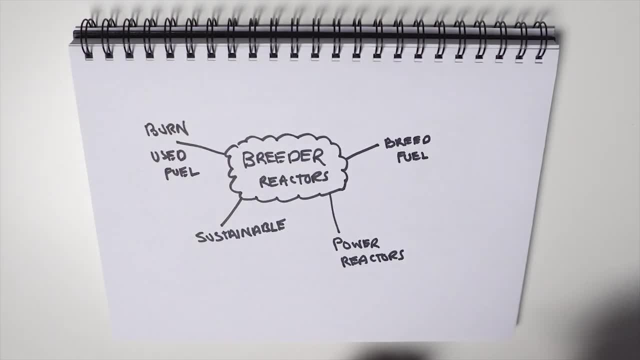 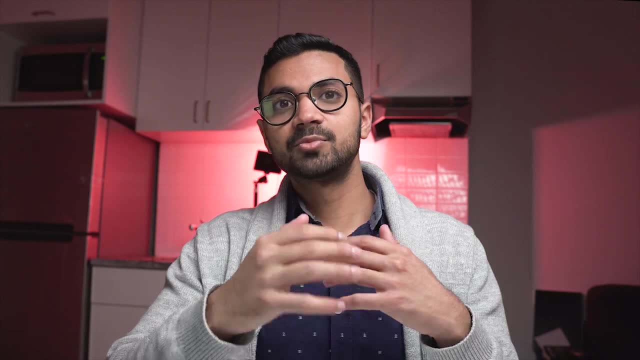 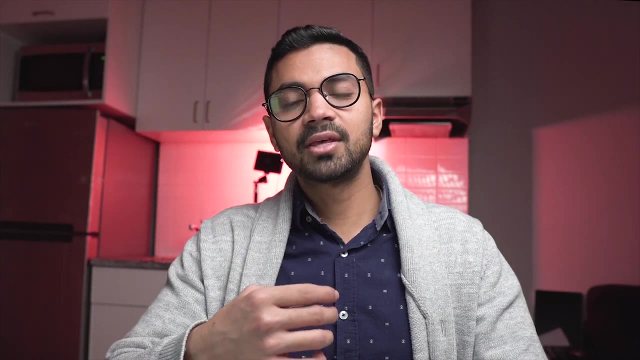 even burn used fuel. Okay, so interest in this technology pretty much died out very quickly because of large uranium reserves that were found throughout the world and also advancements to the enrichment process. But there are operating reactors- breeder reactors- across the world, and it's something that 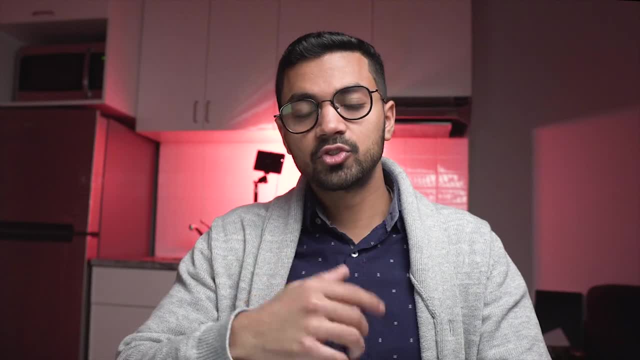 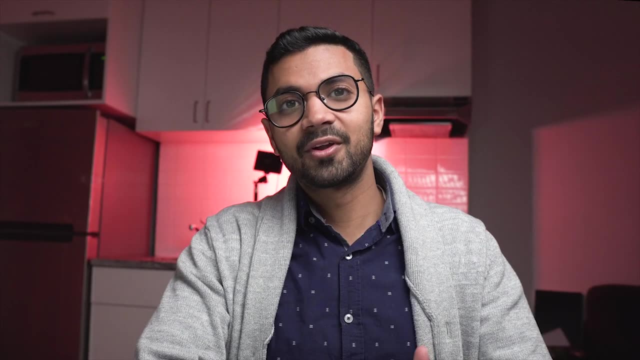 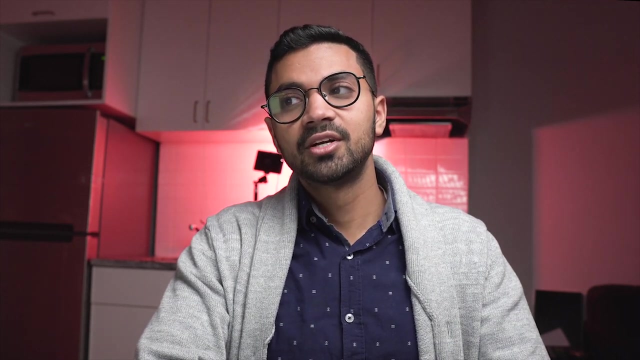 can really close the nuclear fuel cycle in the future. Number three: research and test reactors. like I said, nuclear reactors don't only produce power. Okay, they are also used as neutron sources for experiments, Now, research reactors or test reactors. they don't actually produce energy, so they don't have that turbine, they don't. 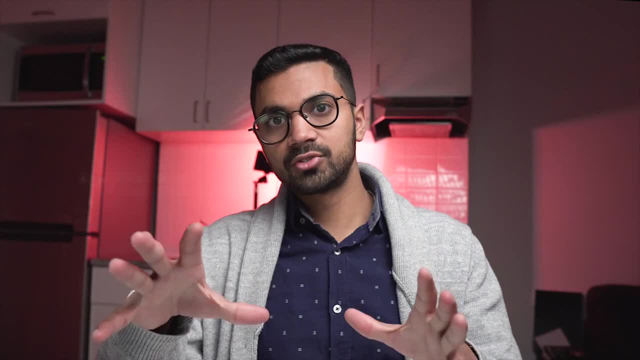 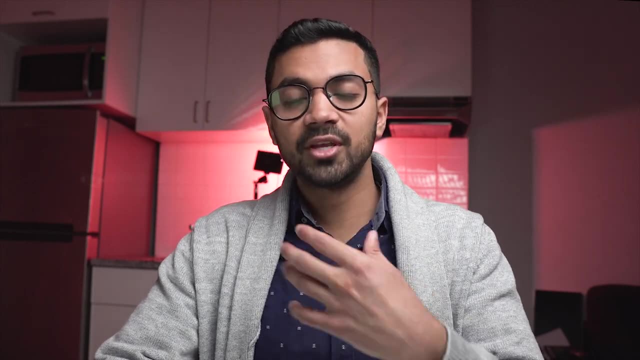 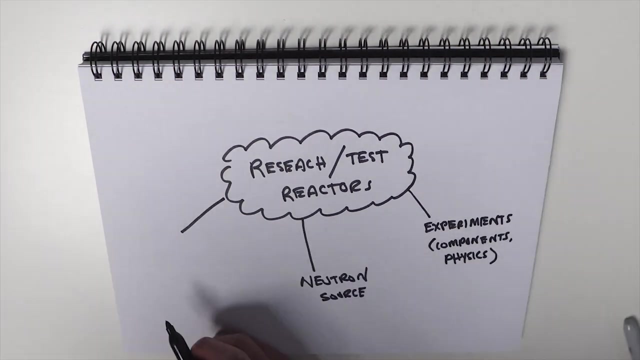 produce steam. rather, they're just a neutron source. These can be found across the world at various university institutions, So universities, master students or PhD students do a lot of testing when it comes to research and test reactors. An example of this is the NRU. 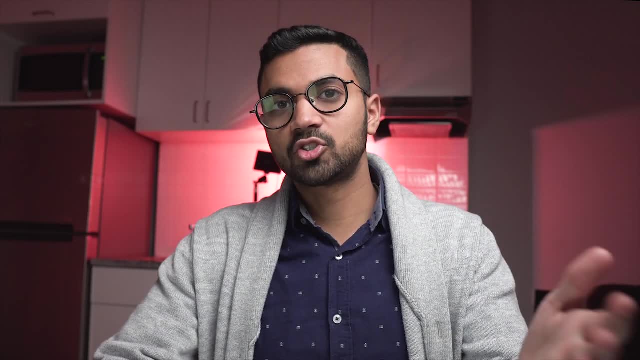 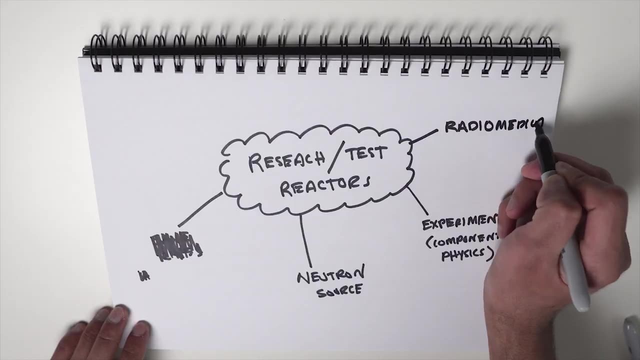 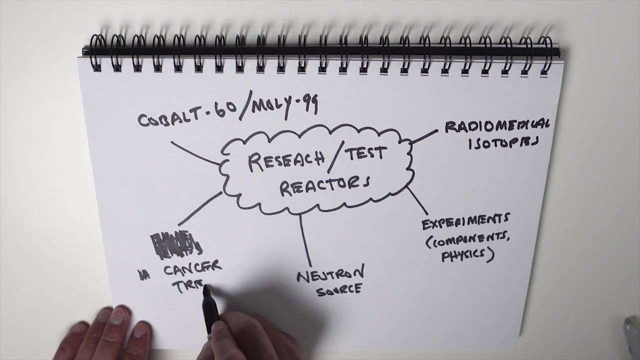 National Research Universal Reactor based at Chalk River. It's used to test fuel bundles. It was also used to produce radio medical isotopes. Okay, it was once used to produce almost 40% of the radio medical isotopes for cancer therapy and 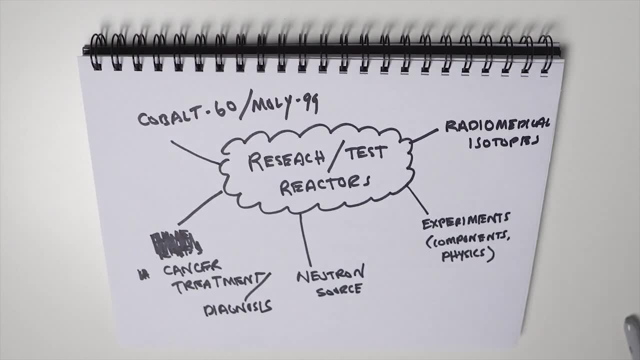 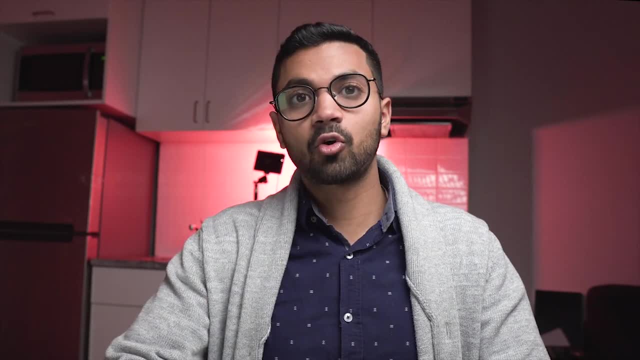 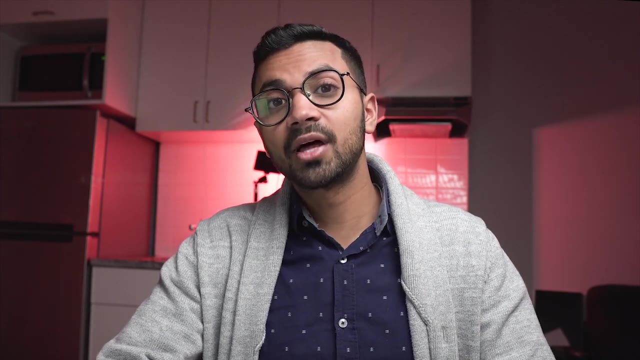 diagnosis across the world. Okay, so these reactors save millions and millions of lives across the world. Some of these medical isotopes that they produce are cobalt-60.. Cobalt-60 used is used for cancer therapy and cancer diagnosis, and also molybdenum-99, moly 99.. Power: some power reactors are also used to produce radio medical. 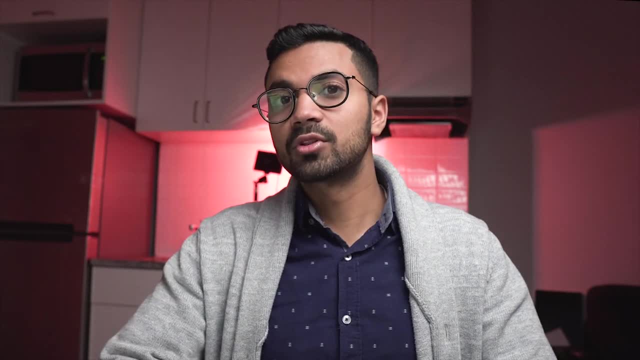 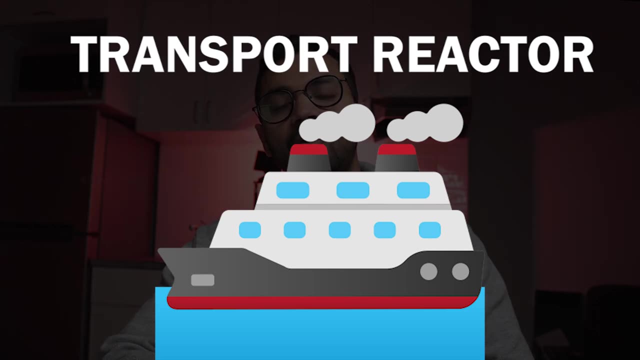 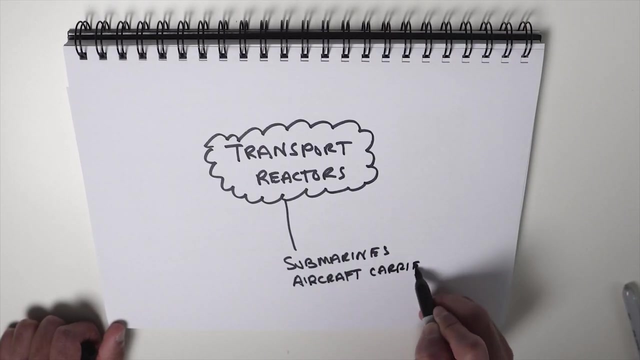 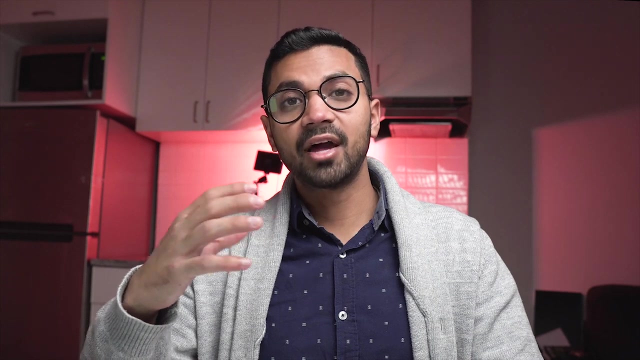 isotopes, such as the can do Canadian deuterium nuclear reactor. Number four: transport reactors. Transport reactors are interesting because they are perfect for Marine technology: Okay, submarines, aircraft, carriers, icebreakers. So the reason why these reactors are perfect for Marine transport is because of the advantages that they provide, such as ability. 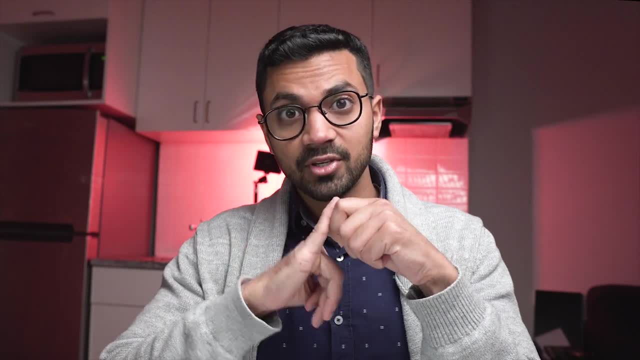 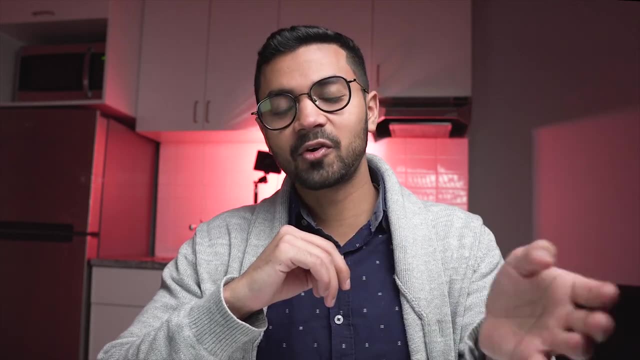 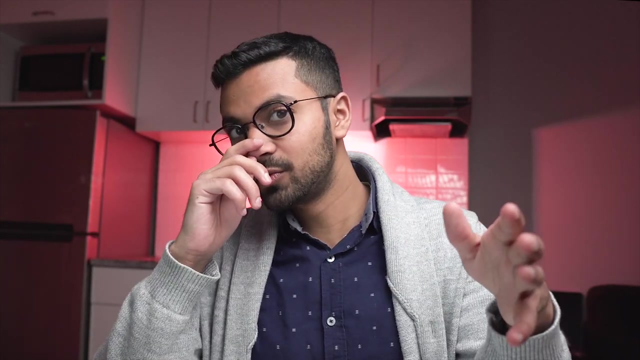 to provide huge amounts of energy for propulsion of these vehicles. Number two is you don't have to refuel them every so often. like a gasoline-powered car, Nuclear fuel lasts long, long times, Sometimes several years, before you need to refuel, right? What's different about these reactors is: 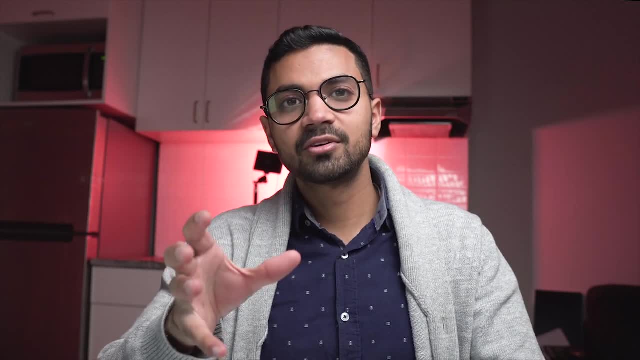 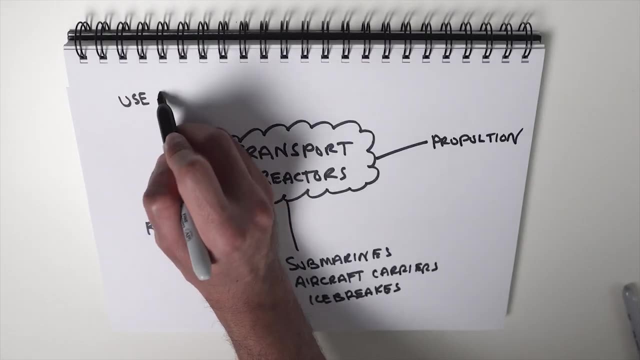 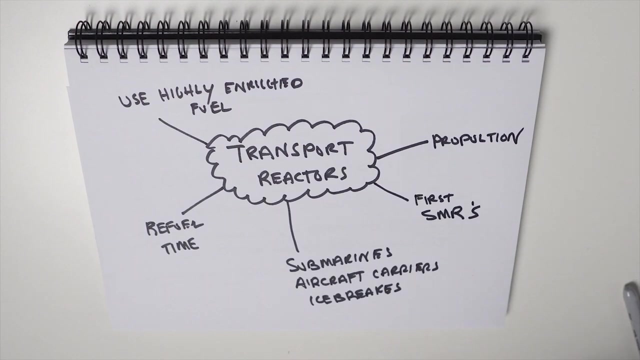 that, instead of using four to five percent enrichment of fuel, which is used in conventional nuclear reactors, power reactors, vehicles, these transport Technologies use a very high level of enrichment, around 80 or above, and they are also the first examples of smrs, small modular reactors, factory-built reactors which drive down costs. 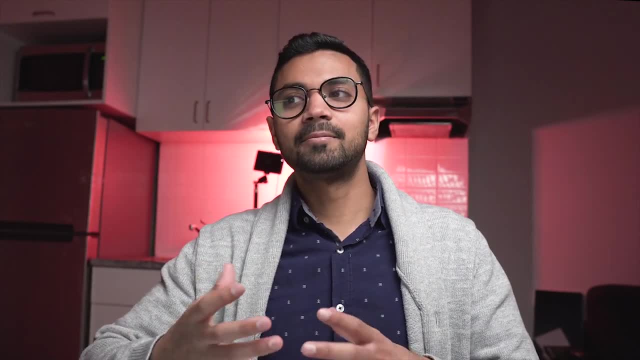 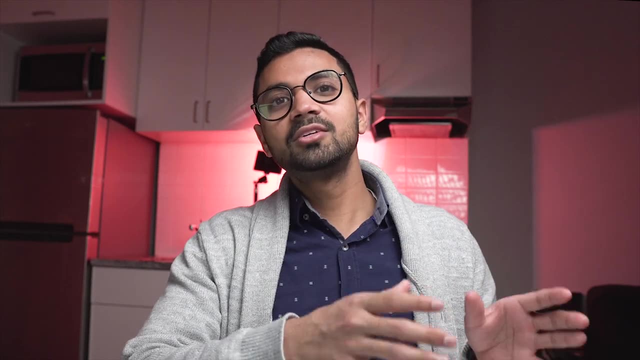 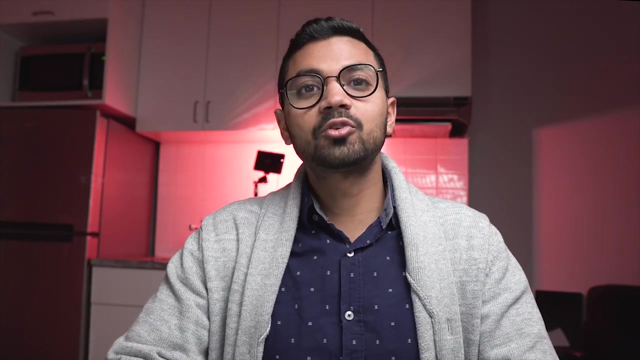 and allow for a simplistic design. This is a technology which is actually being explored across the world, For example, implementation in off-grid communities, rural Arctic communities or simply even being used in cities. So there you have it. Those are the four types of nuclear.